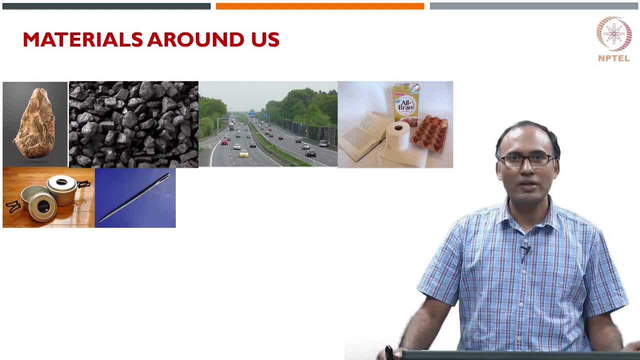 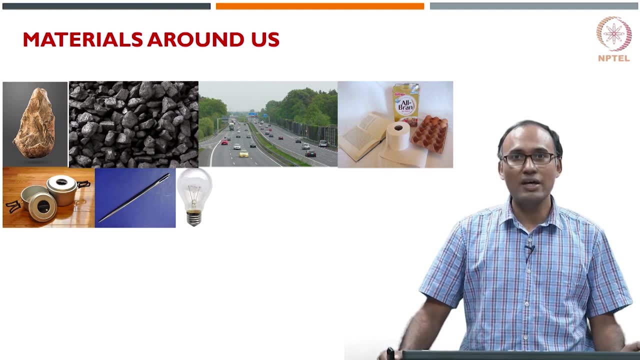 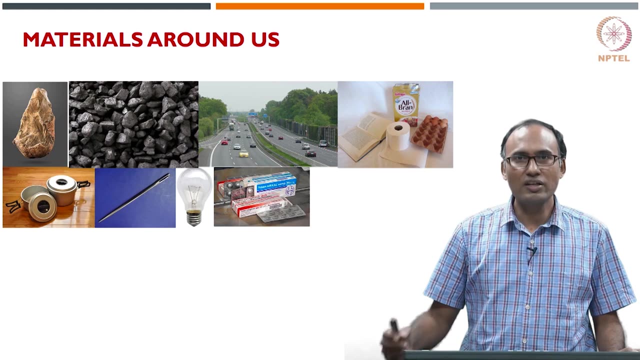 And several other materials, like utensils for cooking needles and even for electricity, that tungsten filaments that are used in electric bulbs and the glass and so on, And even for when you come to health care industry. the pharmaceutical industry relies on the different. 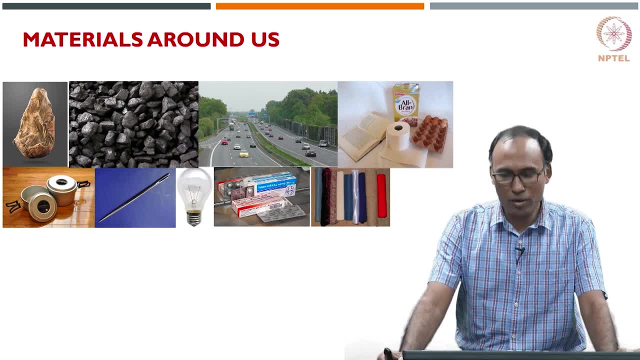 kinds of materials and, important thing that we are not really aware of, the fact that we use lot of textile. Very important It does, pardon, Otherwise will give you unserious problems, But what where our cyber证 Key to the Naruto brain? that is just to increase the monitoring of about. 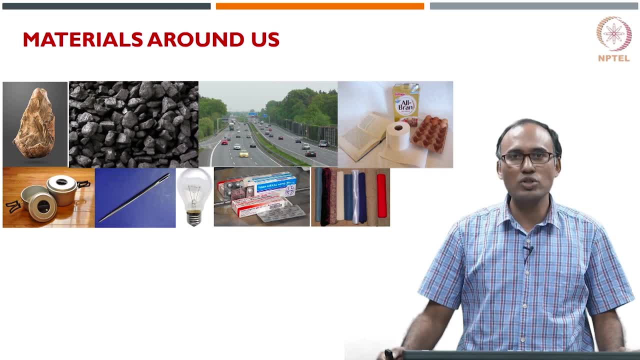 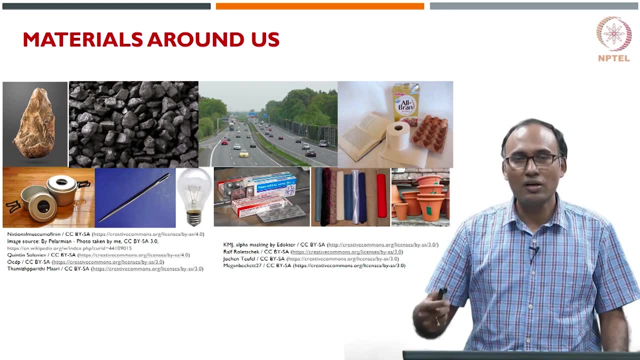 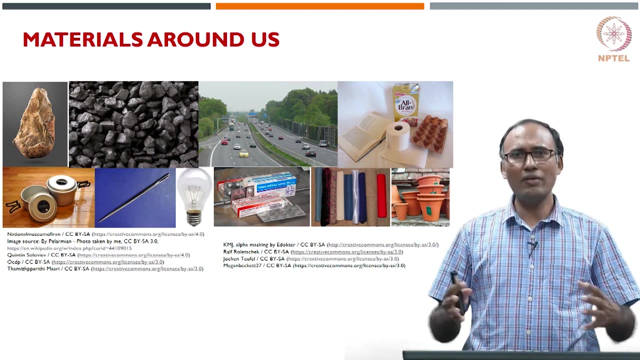 of textile in our daily life and that forms one of the most important materials that we use on daily basis. and, last but not least, the earth, earthen pots, which we are using from ancient times till date. right, So, if you see, I have only given you few examples, but if you see, if you imagine, you can think. 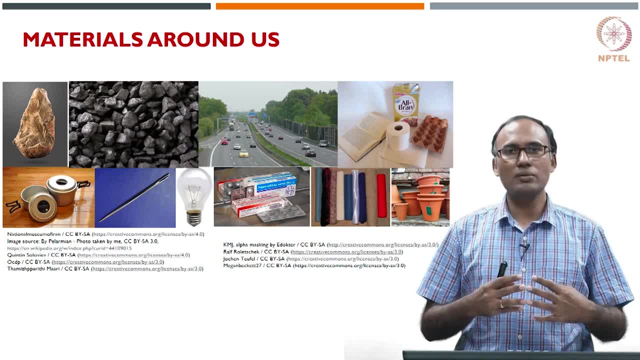 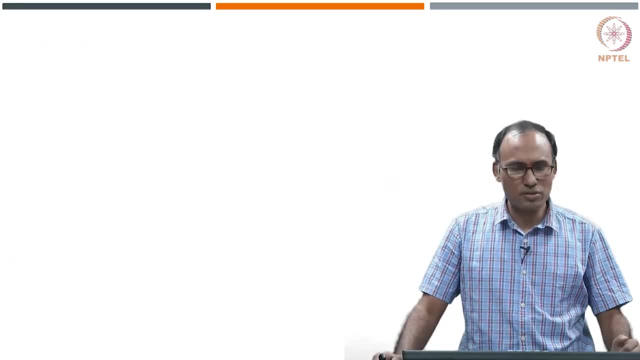 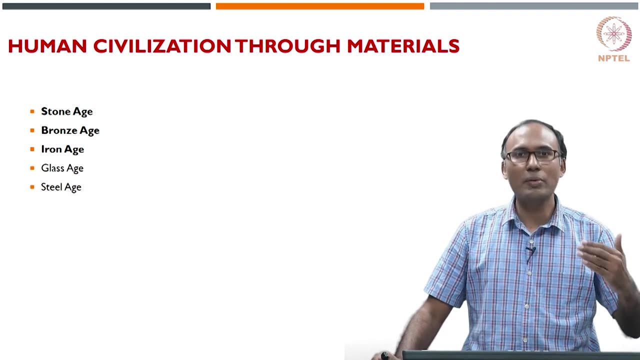 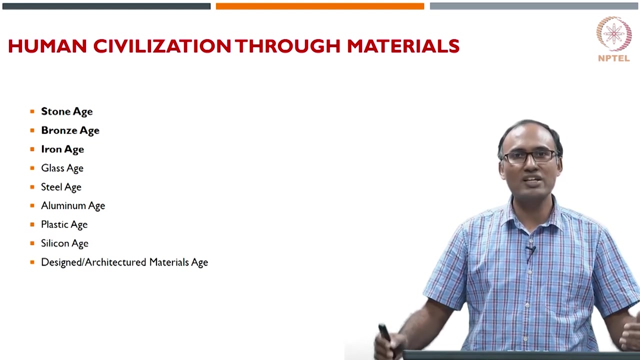 of any system. you cannot think of the system without the materials, say in there, right? So how even human civilization? if we think about the evolution of human civilization, that also starts from the materials. right, even the classification of human civilization is done as stone age, bronze age and iron age. 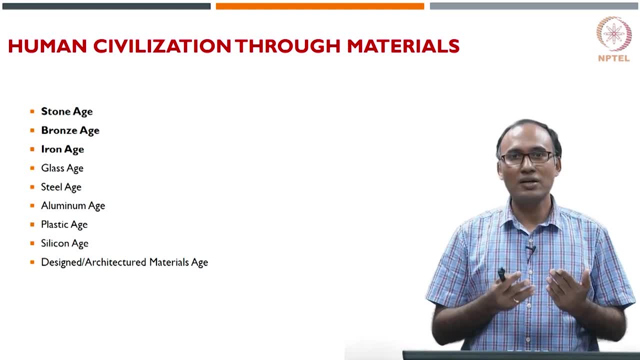 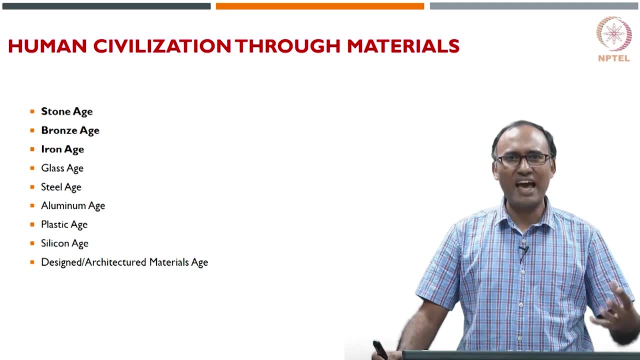 So, basically, the materials forms the basis for the definition of our life, Of our civilization or evolution of our civilization, and we can see several other types of materials like glass, metal, steel, aluminum, and the new age materials like designed and architectured materials, right. 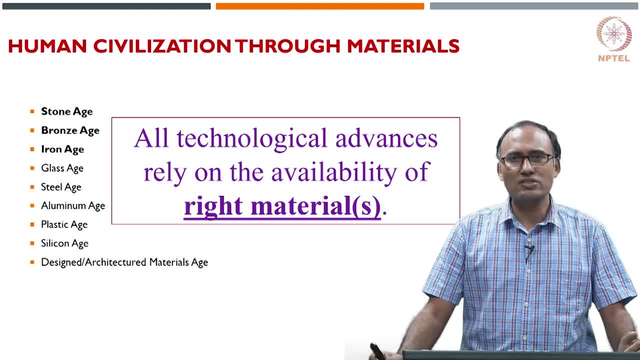 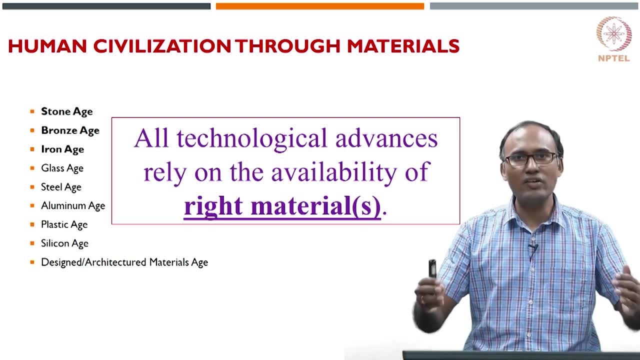 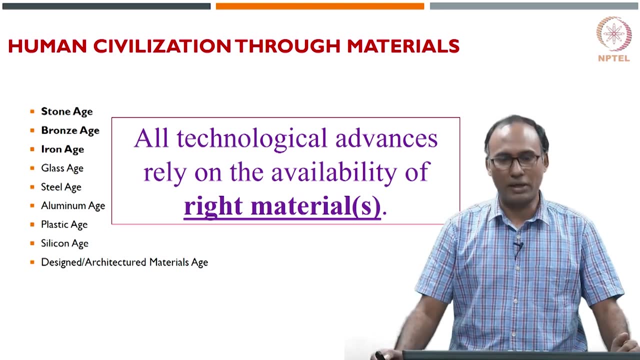 So, in a nutshell, all the technological advances that we are seeing today or we are going to see in future rely on the availability of right materials. until the advent of right material, you would not have made that technological jump, or technological progress, so to say. Alright, so the potential audience for this course, or undergraduate students of engineering. 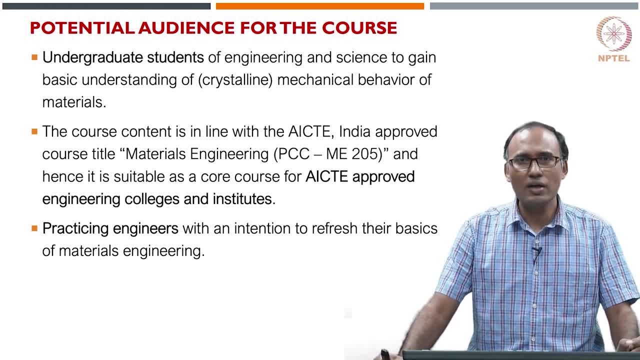 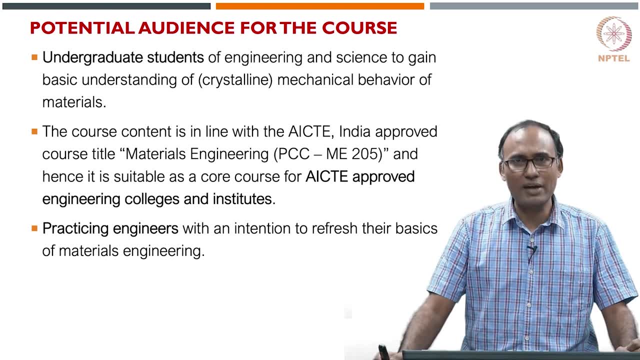 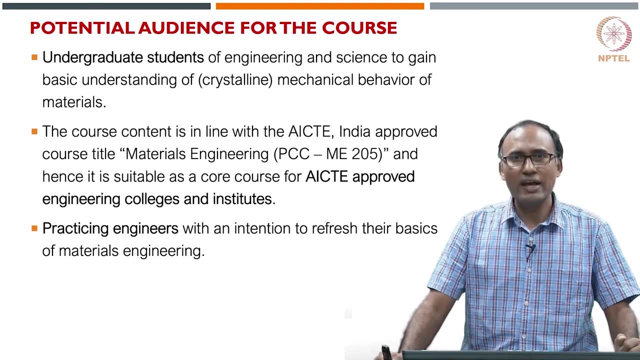 and science, primarily in their forth or fifth semesters. So its the course may be interesting to the students of mechanical engineering, civil engineering, aerospace engineering and other allied branches of engineering. okay, So the content of this course is aligned very much with the AICTE approved course on materials. 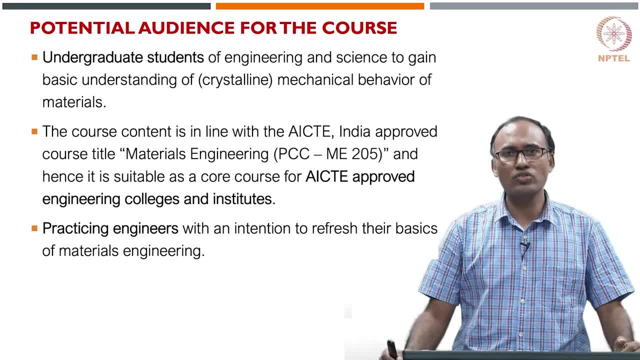 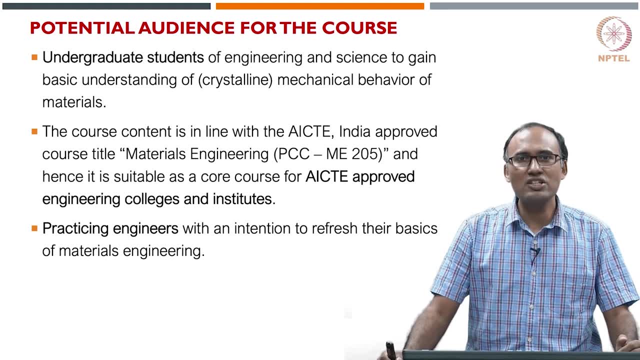 engineering and hence this can also form a as a core course for engineering. So that is what I am going to do, Ok, engineering colleges around India which are approved by ASCE, and the course can also be interesting to practicing engineers who wants to brush up their 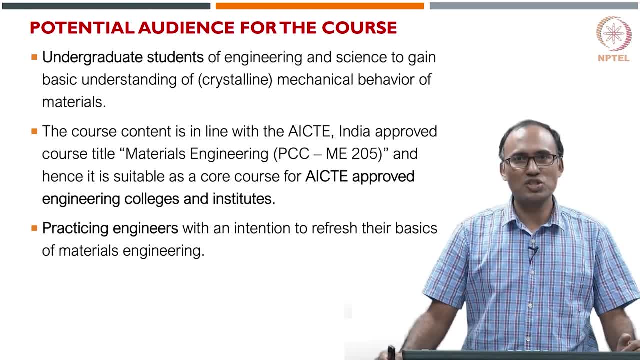 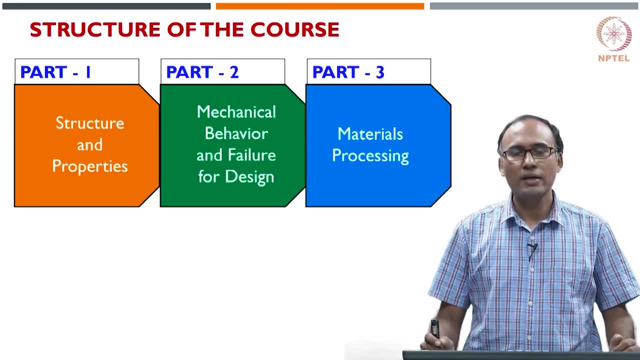 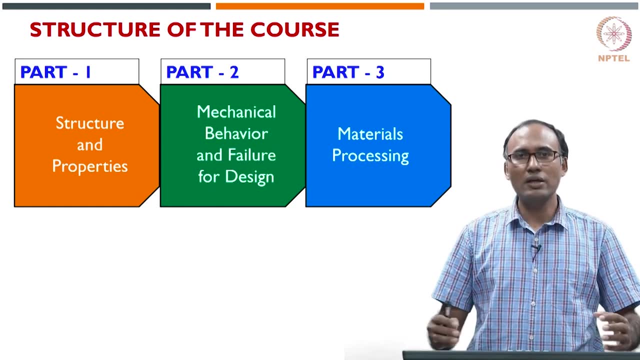 fundamentals of material properties and their structure. so the structure of this course is based the straw is designed in three parts. the part one deals with structure and property of the materials and part two deals with the mechanical behavior and from there we will try to understand the failure of the way. 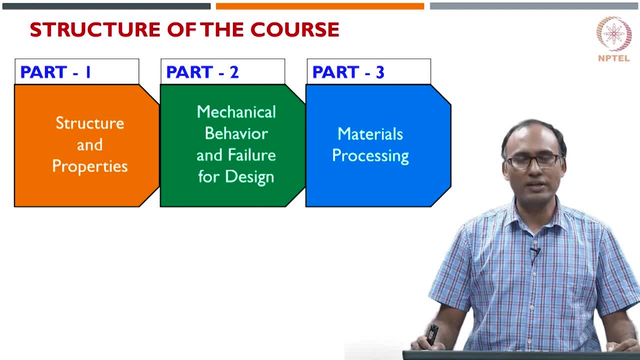 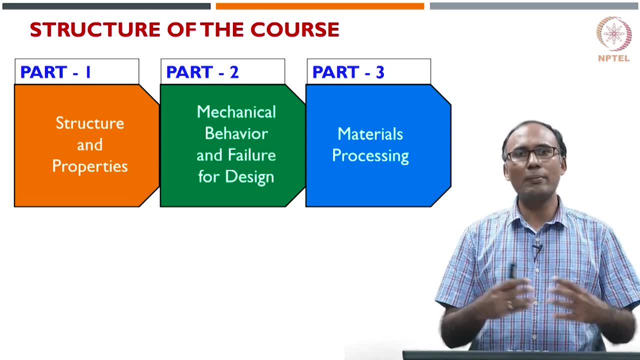 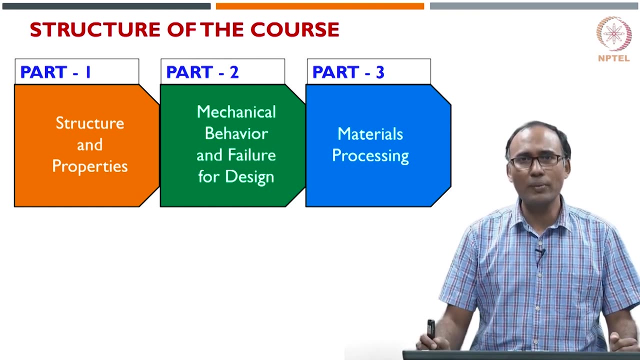 materials for the design of components, both for mechanic primarily. we will may we will be focusing on mechanical engineering components, but the principles that we discuss should be applicable for all branches of engineering as far as failure analysis and design is concerned. and the last and final part is going to deal with material processing, wherein we will 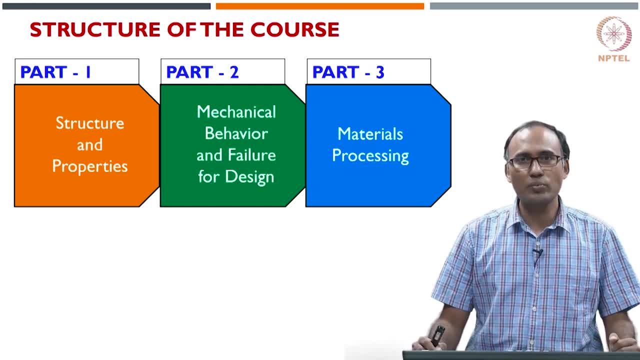 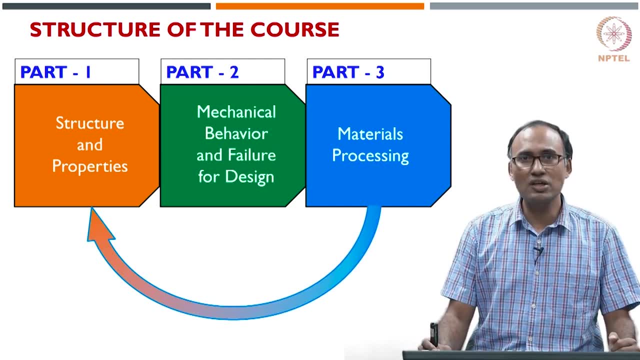 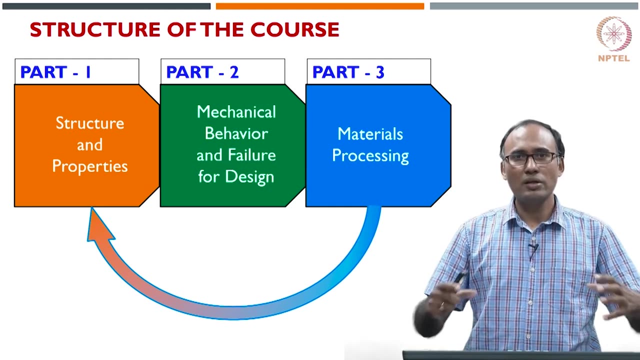 study how different material properties one can use to design the material and how it can be used to design the material can obtain by different processing routes, and then we will see how this processing leads to a particular structure and the ensuring property that is obtained through this processing. so in these three parts will sort of give 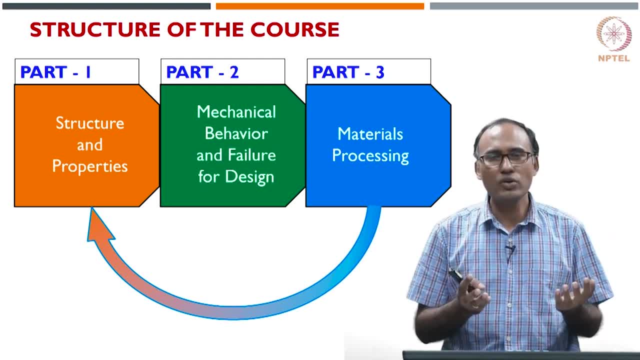 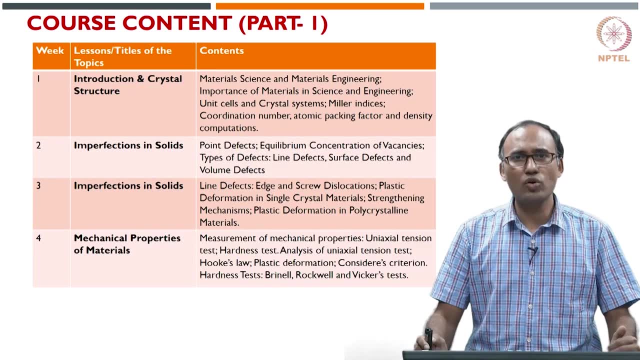 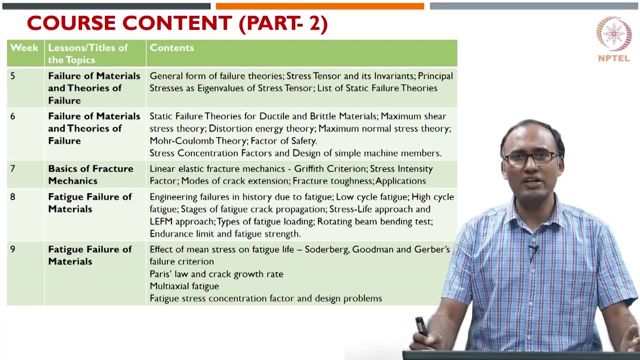 us very fundamental understanding, a basic understanding of materials which can be used for later courses in your branch of engineering. so the detailed contents of this course for each part: part one primarily deals with structure and property and part two deals with mechanical behavior and failure, and we will discuss the failure theories both for static and dynamic loads and in the third. 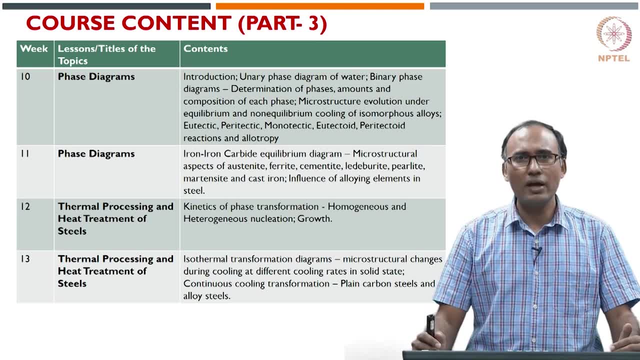 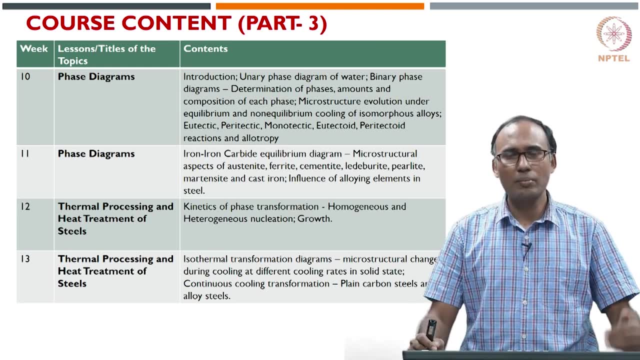 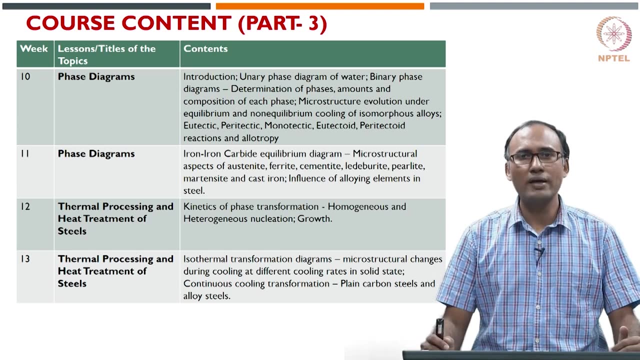 part, we will be primarily focusing on binary phase diagrams and we understand, try to understand, the evolution of microstructure during solidification, from a liquid state to solid state, and we will also spend some time understanding iron- iron carbon equilibrium diagram, followed by thermal processing and heat treatment of steel. 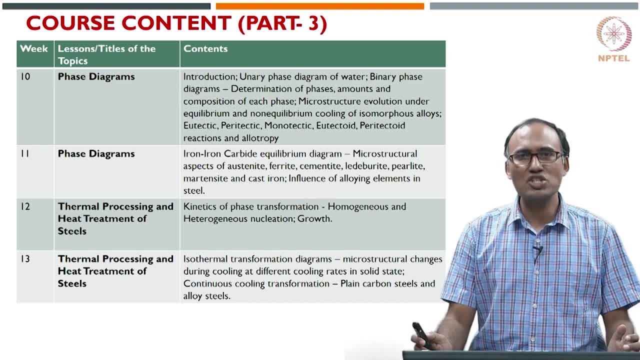 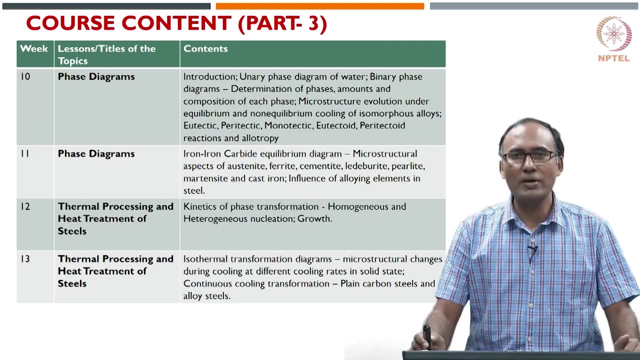 So with that we sort of get an understanding of how material processing will lead to a certain structure and which will further lead to certain properties that we would like to have for components of our interest. So the text books for this course, the main text book for this,